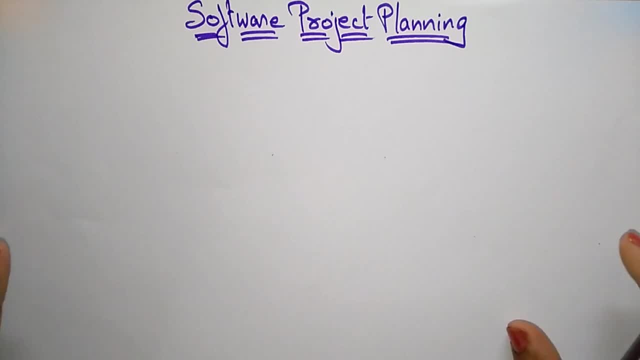 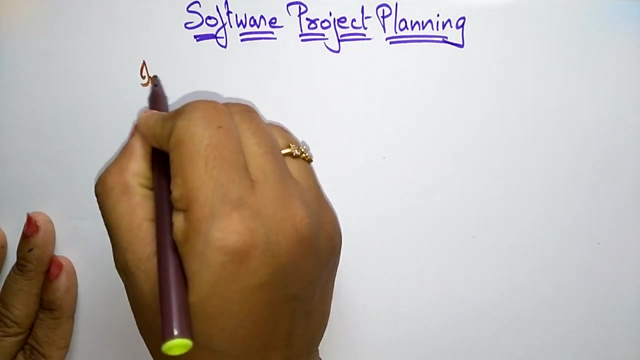 Hi students. coming to the next topic, that is a software project planning. So what is a software project planning? So, if you want to develop any software, you need some planning. That is a systematic planning. Okay, now let us see: In order to conduct a successful software project, we have to understand. Okay, let me write that In order to conduct a successful software project, we have to understand. 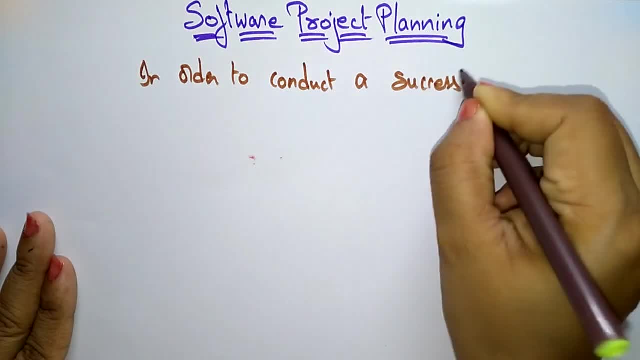 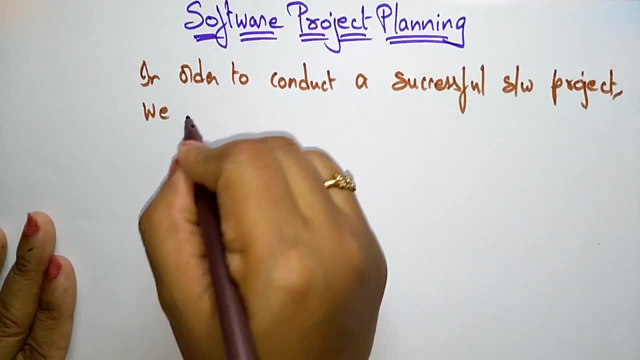 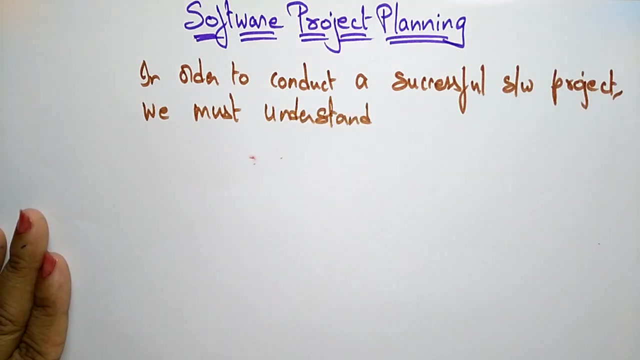 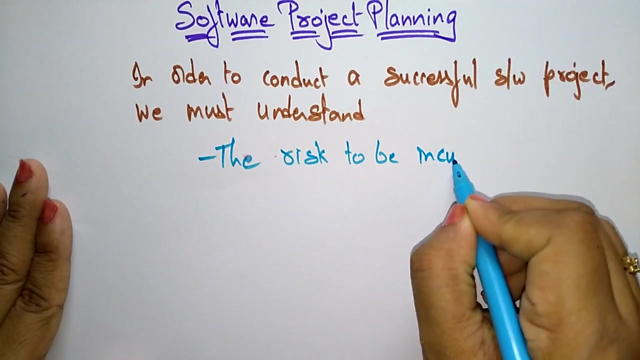 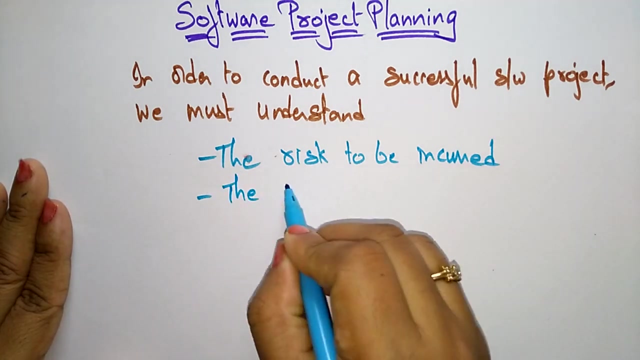 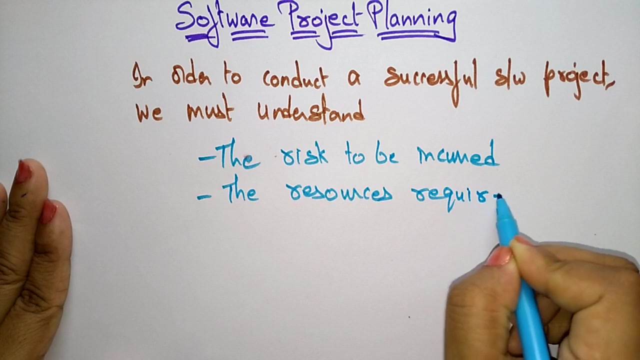 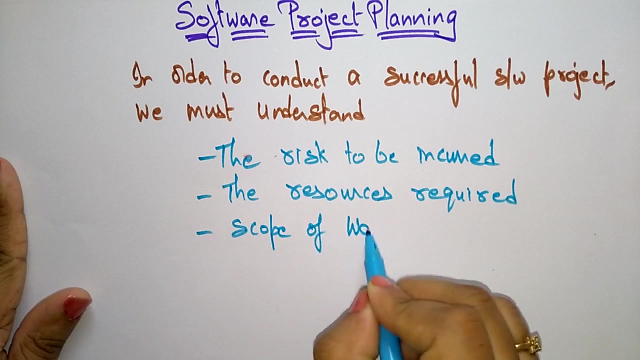 A successful software project, we must understand. We must understand the risk to be incurred. So what are the risks that are present in the software that we to develop the software, that risk has to be incurred. Next, the resource requirement: You have to check what are the resources that are required to develop the project. The resource required, scope of work to be done, Scope of work to be done and the task to be accomplished. 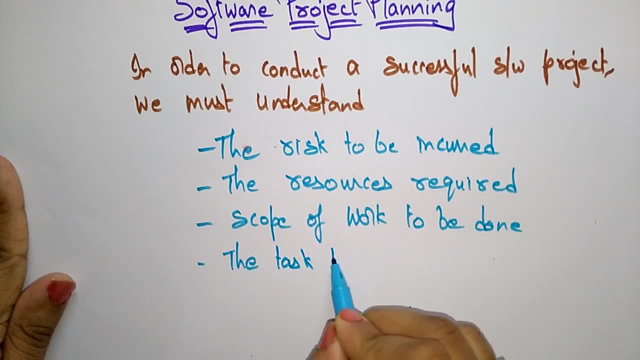 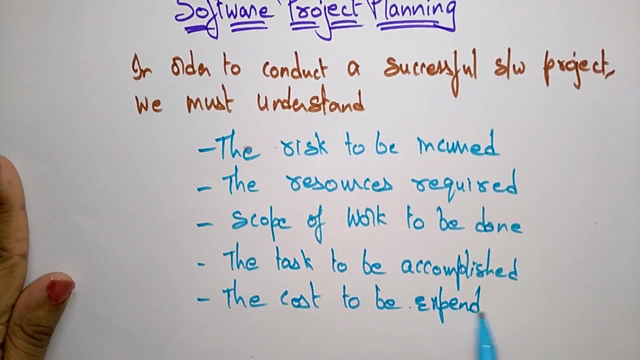 The task to be accomplished, The cost to be expanded, The cost to be expanded, The schedule to be followed, The schedule to be followed. So you have to understand all these topics. So, whatever you want to develop the project in order to conduct a successful project, 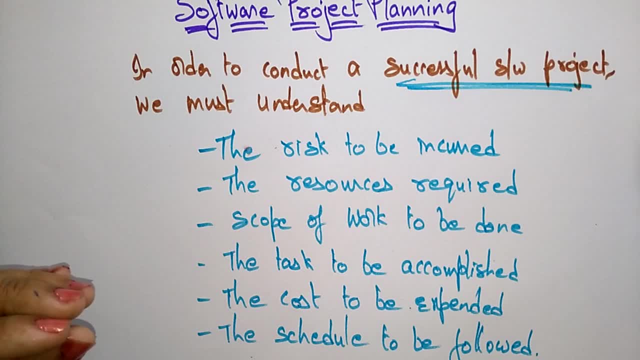 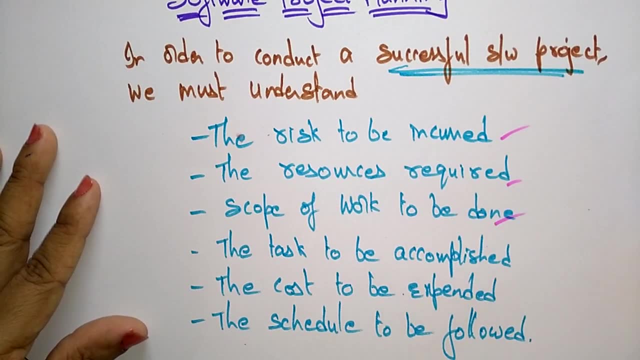 the main thing to develop a successful project. we have to understand what are the risks that are incurred in the project, the resources that are required to develop a project, what is the scope, the lifetime of the project, that work has to be done, the task to be accomplished. 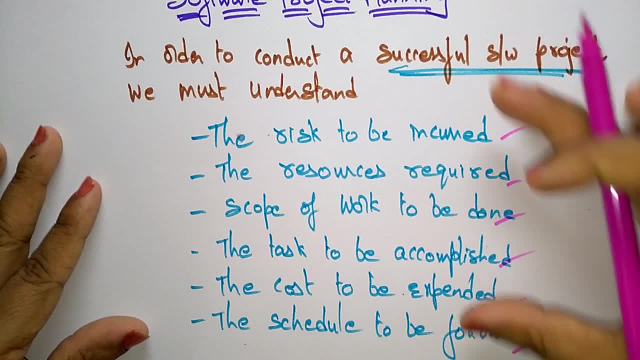 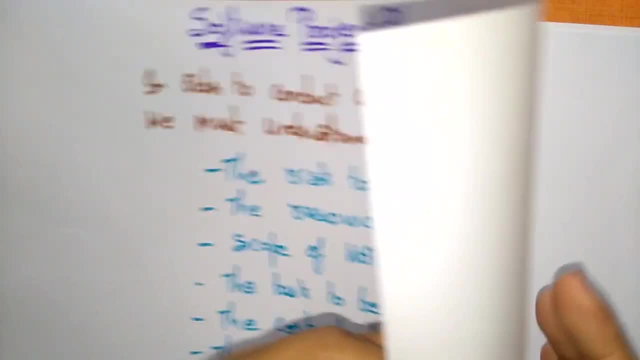 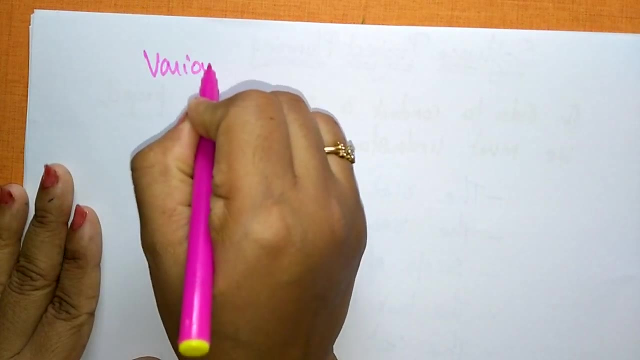 the cost to be expended, the schedule to be followed. So we have to understand all these topics. then we can develop a successful project. So what are the various activities that are involved in planning? Now let me write that: various planning activities. 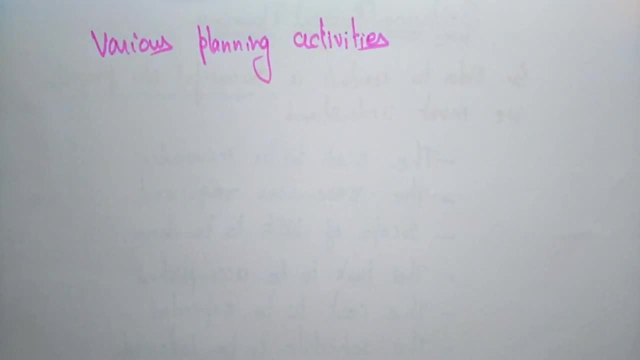 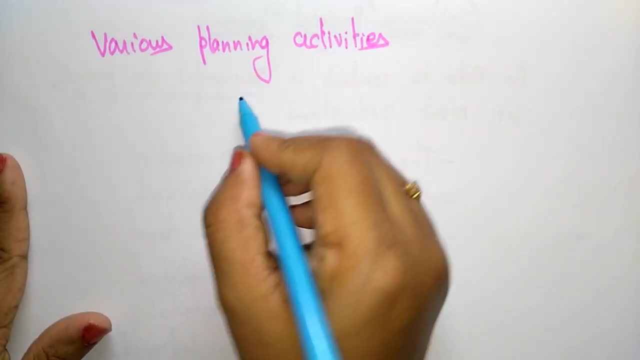 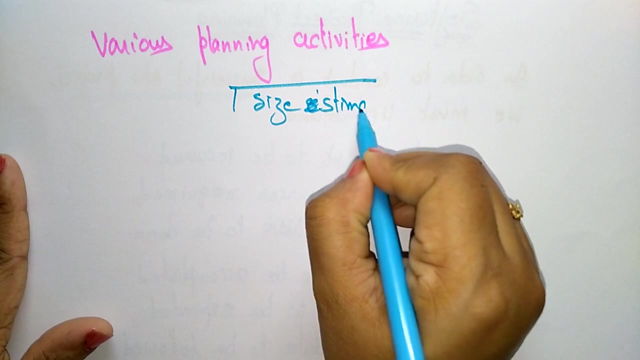 So the various planning activities that are present to develop a project that is a software project. The various planning activities is: you have to know the size estimation, Size estimation, the size estimation of your project. you need to know the cost estimation. 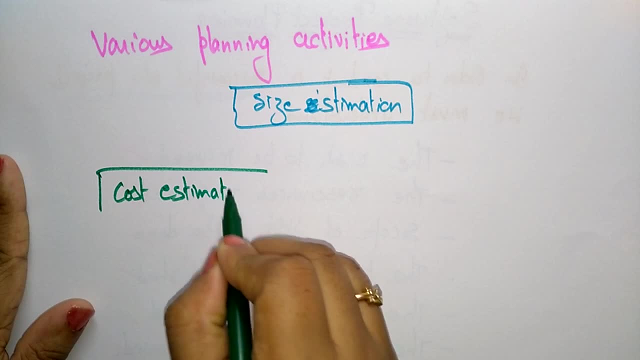 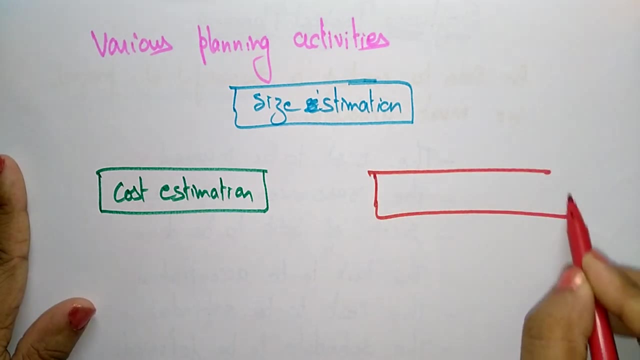 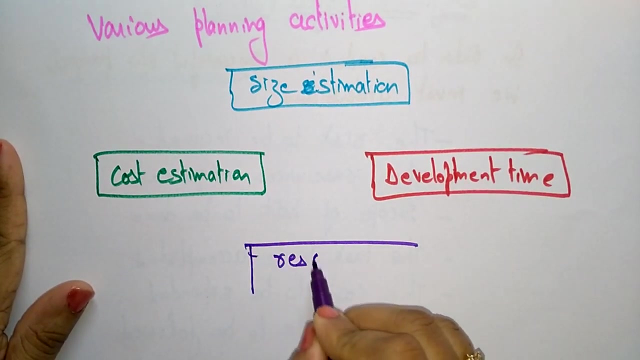 The cost estimation of your project and then the development time that it requires to develop a project: development time, Development time- And you need to. You need to know the resource requirements, the number of resources that are required to develop a project, resource requirement and the project scheduling. 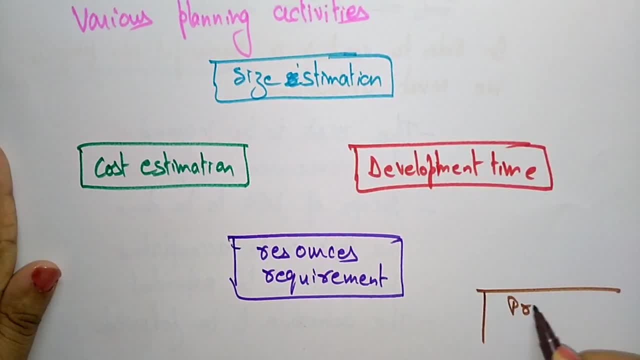 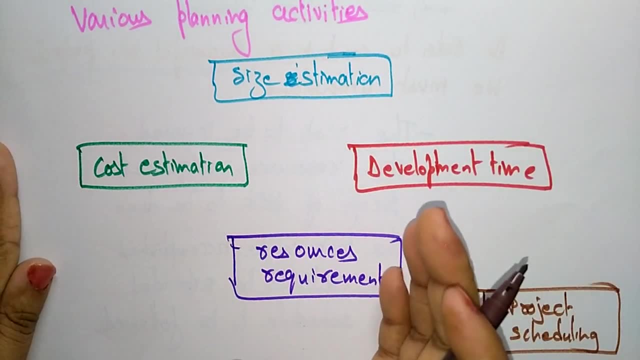 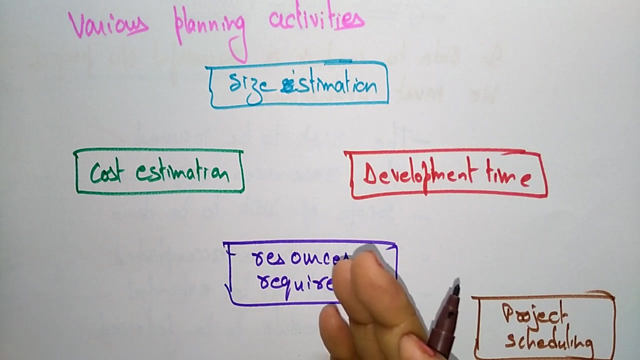 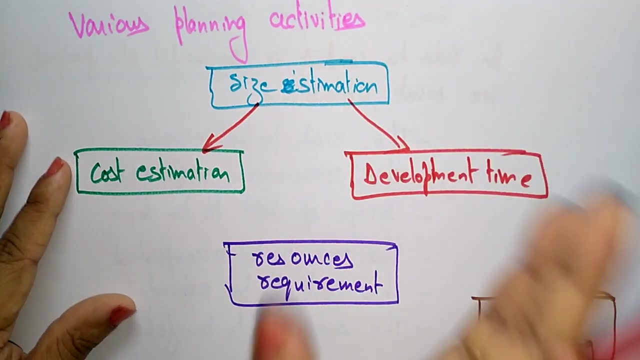 So now let's see. next one is the project scheduling. So these are all the various planning activities. to develop any software project, to develop any software project, You need some planning activities. So the those planning activities are size estimation. So if you know the first, if you know the size of the project means how much line of 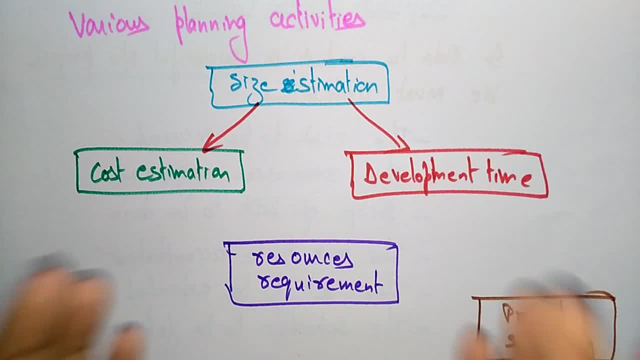 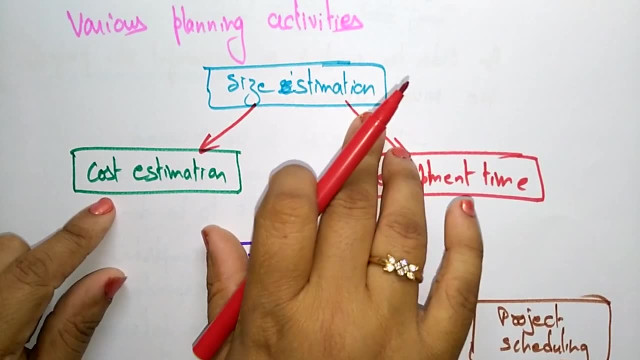 code it is going to be take to develop a project. That is the memory that is occupying. that is occupying to develop a project. the size of the estimation you have to know, And after that you know the size, Then you have to see the cost estimation. 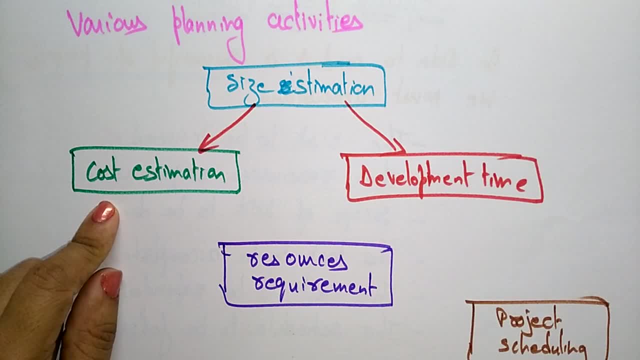 Okay, for this much of MBO, this much of GB, what is the cost of that? Okay, the project: there is a cost estimation and the development time. so if you know that the size of the project that you are going to develop, so you have to calculate what is the development time, the. 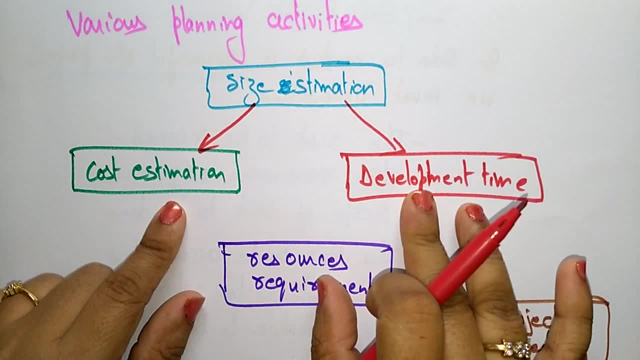 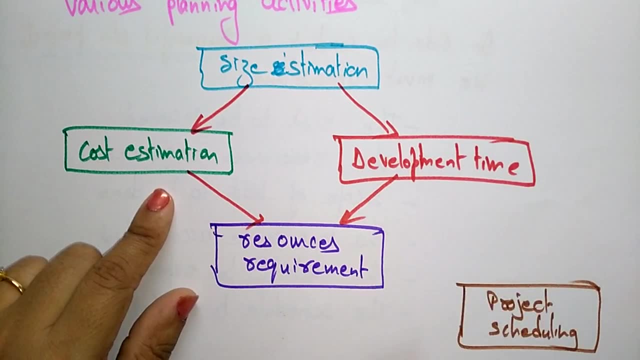 total time that it takes from starting to ending. that you need to know. so, okay, cost estimation is over and the development time we have decided. then you have to think about the resource requirements. so what are the resources that were required to develop a project? so, after that resource,